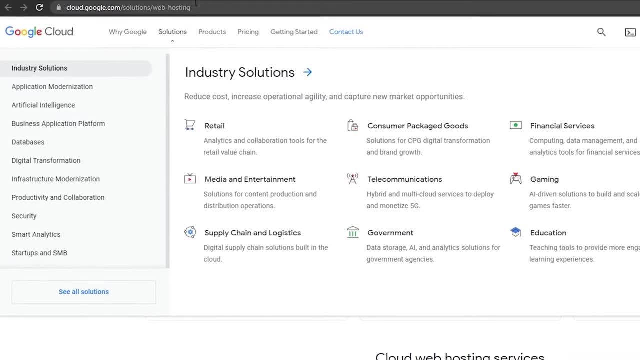 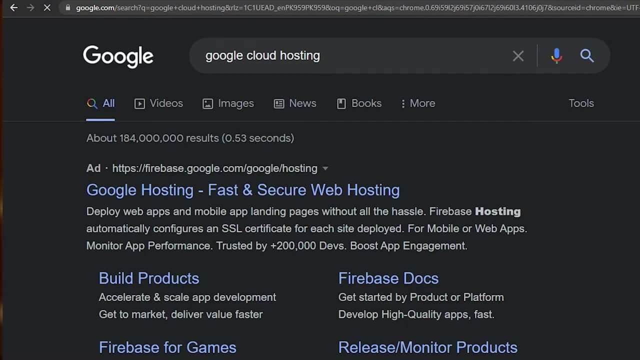 don't see web hosting over here. well then, the process is pretty straightforward: simply open up a new tab in chrome and type in over here: google cloud hosting, and then simply open up the second link, which is going to be this one. so simply open this up and then you will see that. 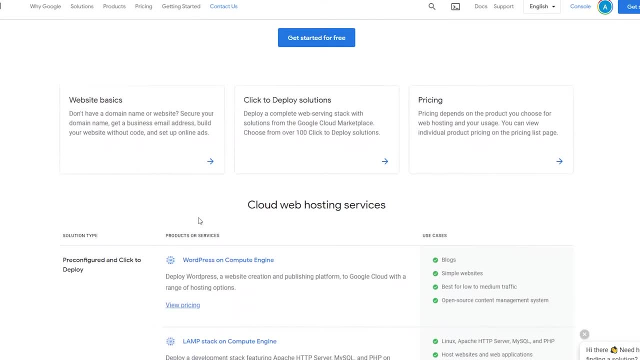 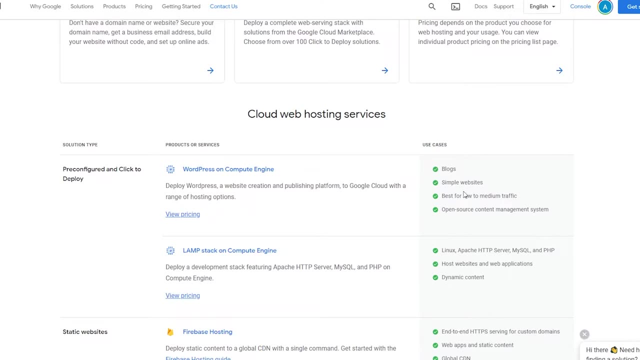 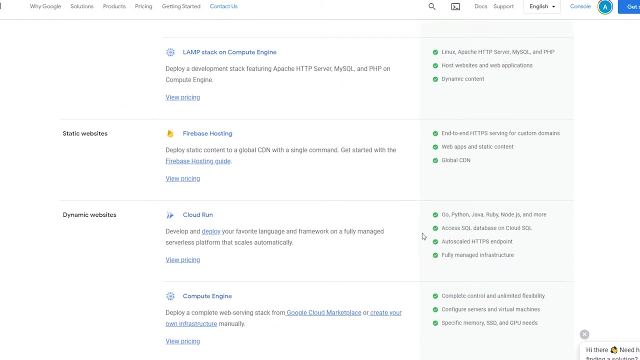 very same page in front of you. so now, from over here, you can basically see some of the use cases of having a free hosting. so you can use it for blogs, simple websites, and also for lower to medium traffic oriented stores or something like that. so again, it all depends upon your computing. 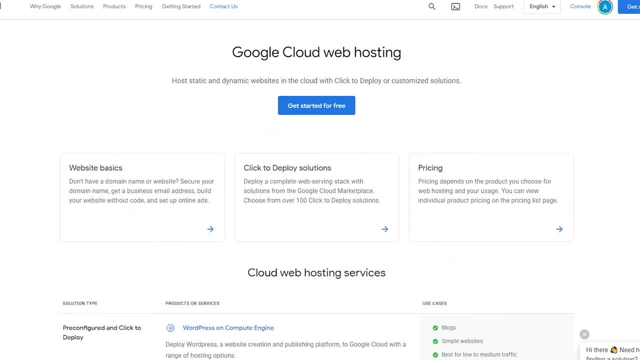 power and your experience. so i'm going to open up a new tab in chrome and type in over here google cloud hosting and then simply open up the second link, which is going to be this one. so simply open and which plan you opt to go for, but i'm going to be showing you a plan which is essentially going to 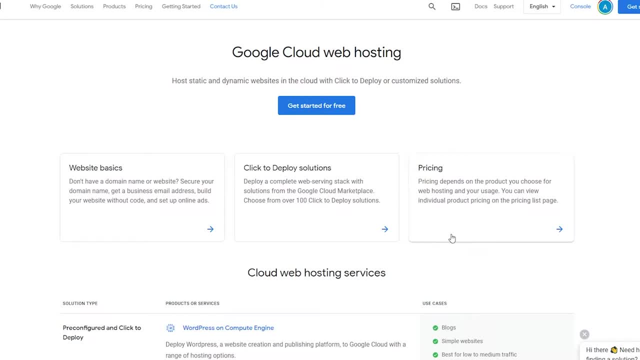 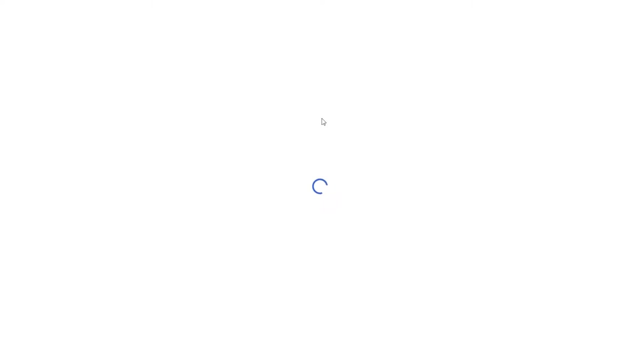 be absolutely free for the first whole month, and even after that it is going to be like almost minimal cost, like nothing too major. so i want you to click on get started for free now and then, simply, from over here, wait for a couple of seconds and then that is going to take you over to this. 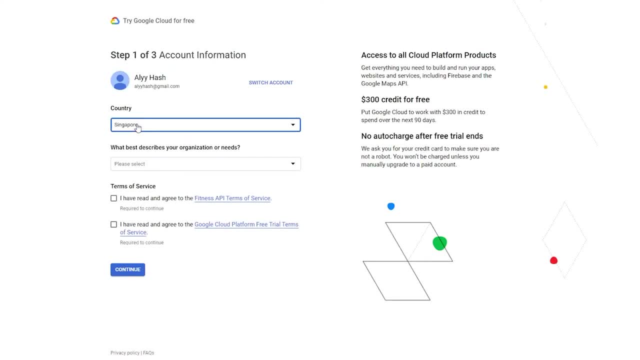 particular page. so from over here, i want you to simply choose your country and also choose which best describes your organization or needs. so simply fill these things out and click on continue, and i'm going to do that right now as well. so i'm going to basically choose my country. 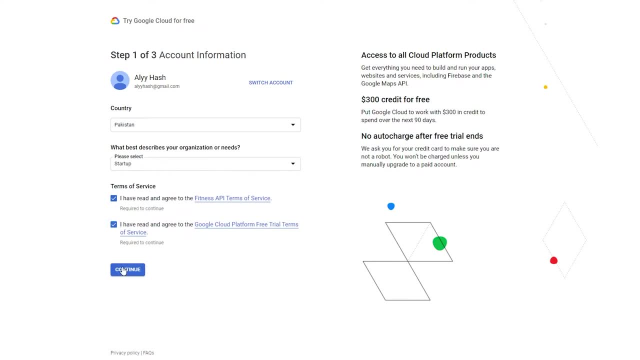 and then also we're going to choose startup this and that, and now i'm going to click on continue. so once i click on continue, i will have to put in my phone number. so i'm going to do that and i'm going to catch you guys in just a second. so once you've done that, now, from over here, 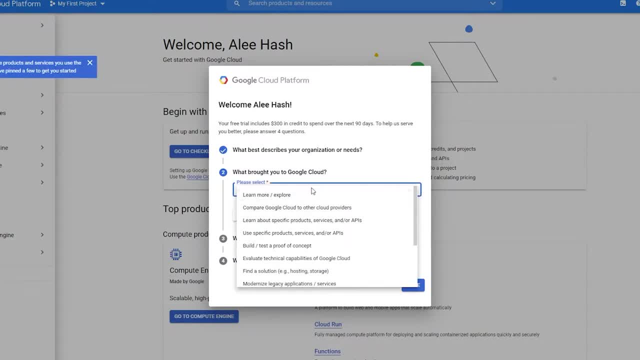 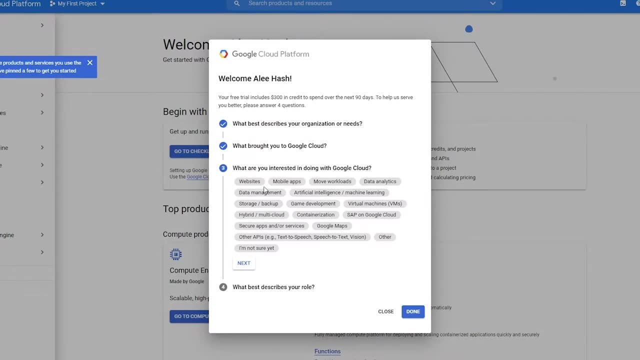 i want you to simply click on these options. so what brought you to google cloud? you can, from over here, choose a video or something so like: simply do that, click on next and then, from over here, what are you interested in doing with google cloud? so i'm going to click on websites and then i'm also. 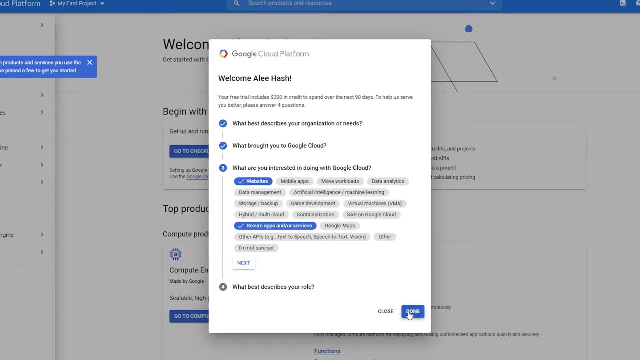 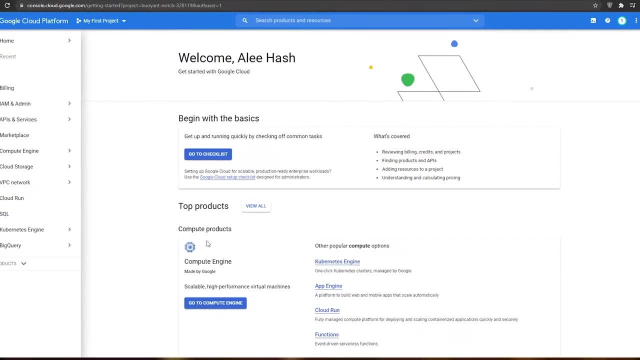 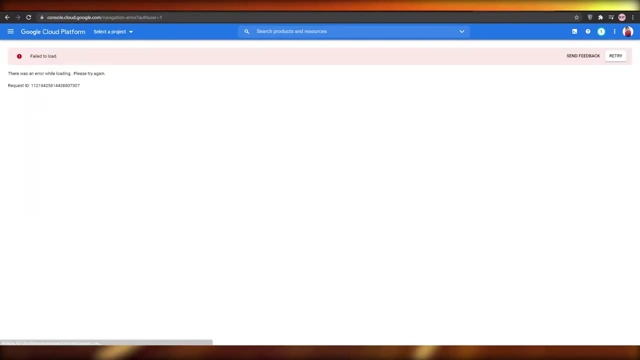 going to click on secure apps or services. so click on done once again. and then there you have it. you have your basic setup in front of you. so now what i want you to do is that i want you to click on go to compute engine. so once you do that, that is going to take you over to this page. so now from. 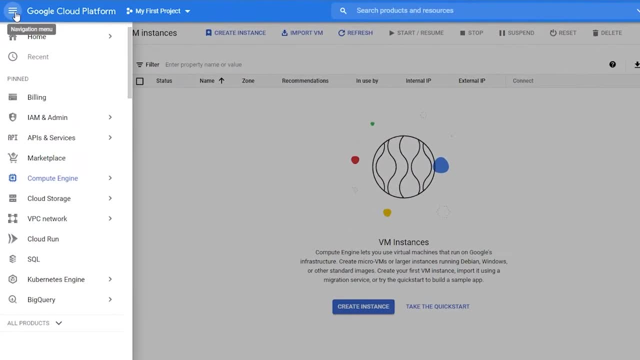 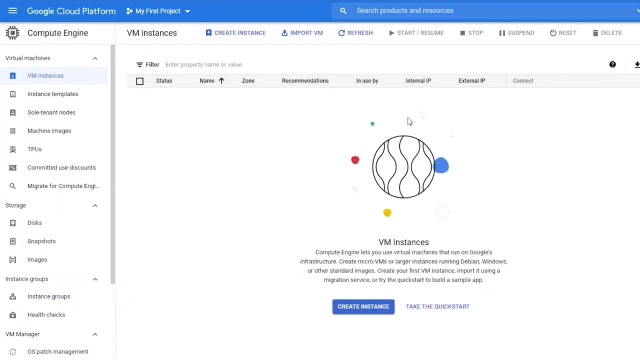 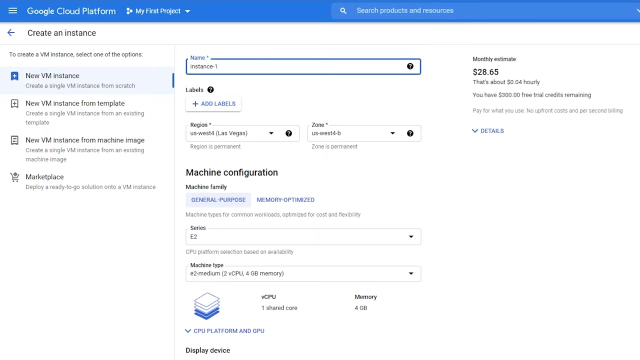 over here. i want you to simply like click on this particular button at the top left, hover your mouse over the compute engine and click on vm instances now. when you do that, you will see this dashboard in front of you. click on create instance and then, from over here, simply give your instance a name. 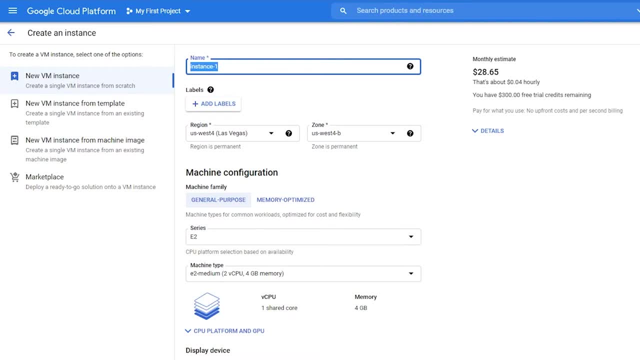 so i'm going to basically give my instance a name and i'm going to basically call it blog personal. so once i do this, well, after that i can choose to essentially add labels or anything. so yeah, like that is up to me, but i'm not going to do that right now. so over here they're saying: 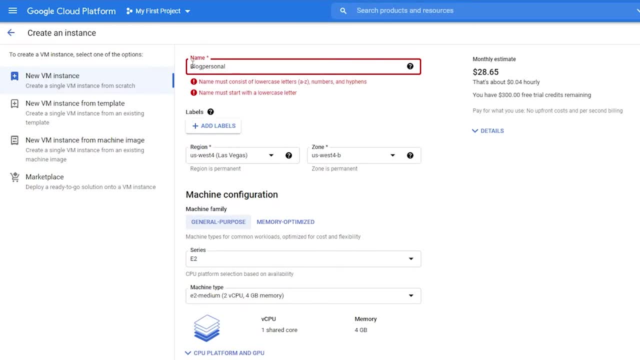 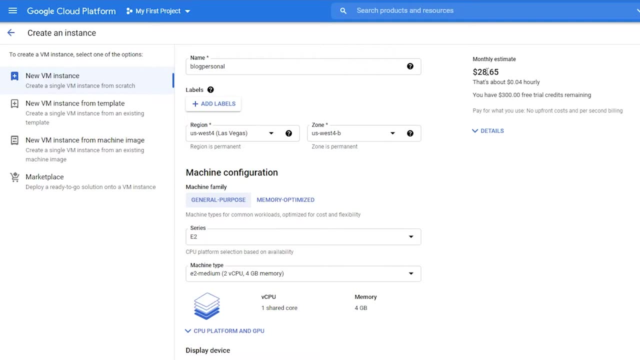 that name must consist of lowercase letters. so i'm gonna lowercase my letters now. on the right side, you will see that they are charging about 30 per month. well guys, you don't have to worry about that, because i assure you we are going to get it down to zero. i mean almost zero, but still it is going. 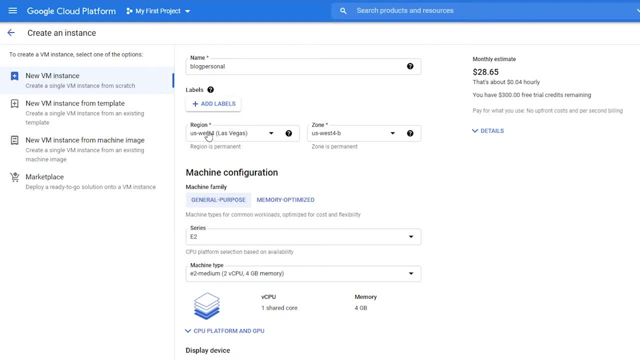 to be free nonetheless. so now, from over here, what i want you to do is choose the region and choose, or basically something that is closest to you. so i'm gonna choose asia, south mumbai, and then, for the zone, i'm just gonna like leave it over here. so now, from over here, i'm gonna choose the computer. 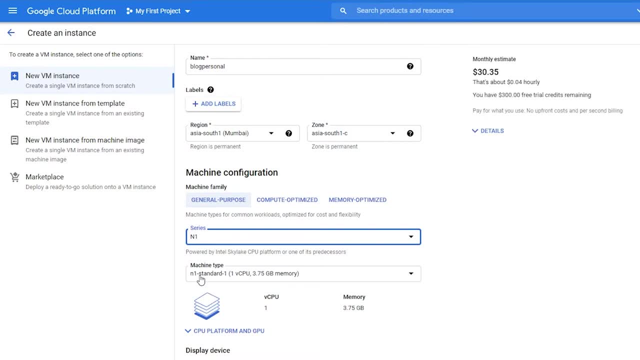 and i'm gonna choose the n1. so once i choose the n1, well now, from over here, from the bottom, i can, like you know, choose different models of the n1 as well. it all depends upon me, but for now we're gonna choose the f1 micro. so once we choose the f1 micro, 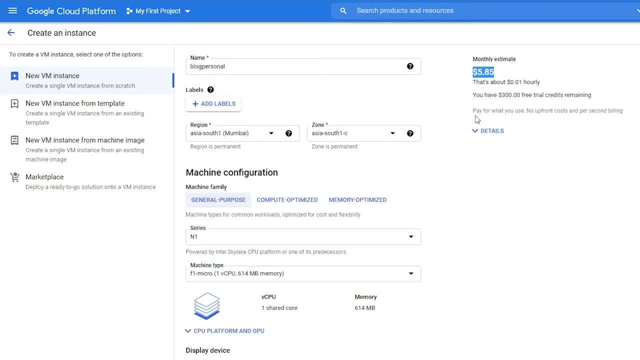 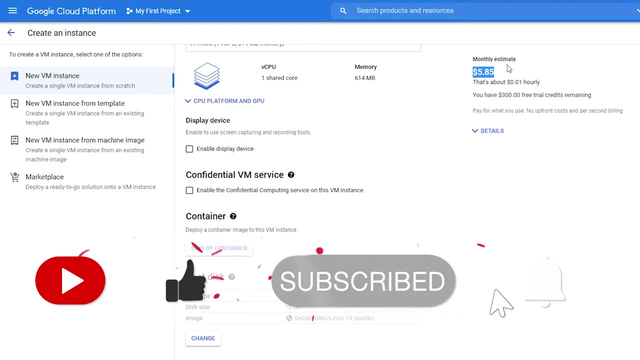 we can see over here that the cost has jumped down to six dollars. guys, that is literally free. i mean like six dollars for like hosting, for absolutely free. i mean that's bad, but still you won't even have to pay the six dollars as well. i mean like this is gonna be completely free. 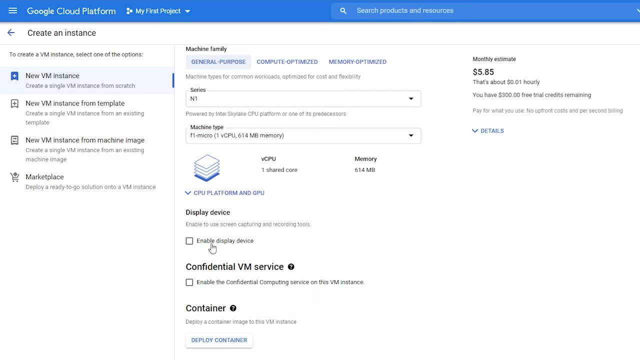 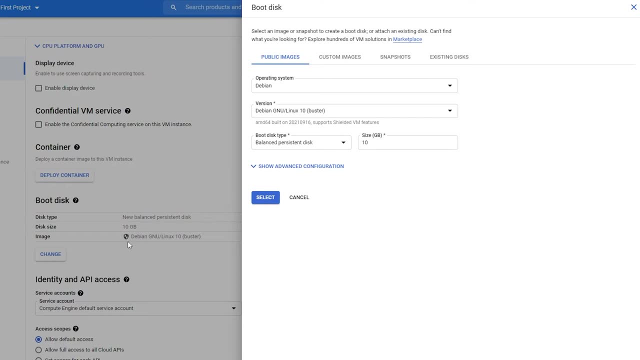 so from over here, you can essentially, like you know, choose a display device as well if you want one, or simply, from over here, choose the boot disk, click on change and then, from over here, simply choose the operating system to be whatever you want. i mean, like, choosing any one of these is not gonna add a whole lot to your cost, so you are going to be. 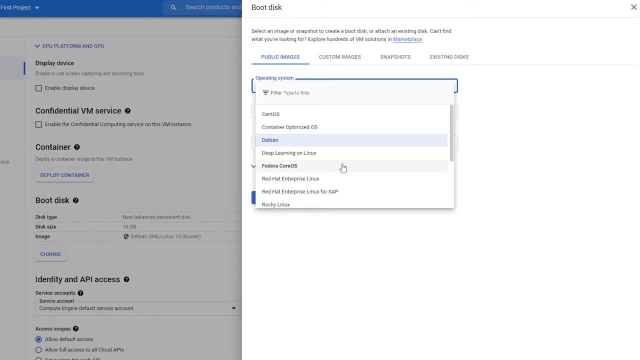 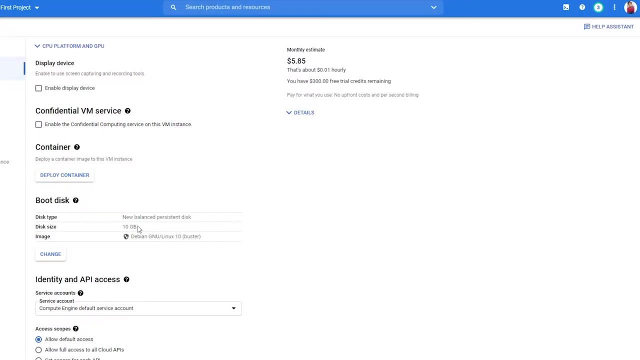 better off either way. so, like, don't worry too much about, like you know, jumping the cost, because it is not going to matter a lot. so i'm going to choose a windows server and then i'm going to basically choose, um, a 30 gb, because, if i remember correctly, we are going to be given 30 gb's of free space. 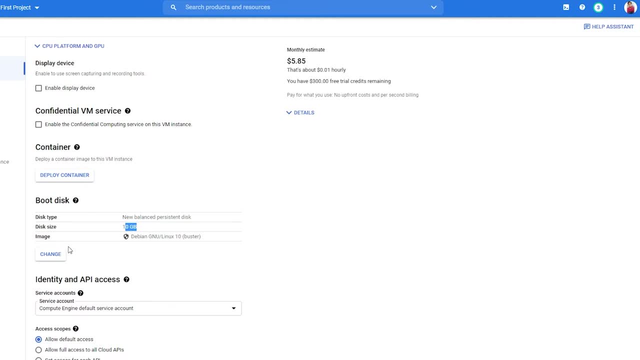 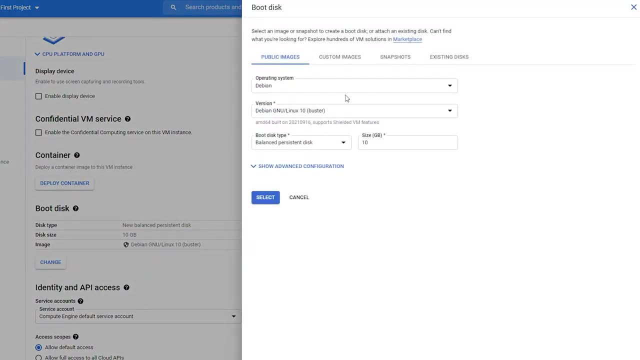 so, like over here, we can see that we are only being given 10 gb's of space, so i'm gonna essentially change that accordingly. so i'm gonna click on change once again and then, from over here again, i'm gonna choose windows and then i'm gonna click on 32, but i don't believe we could get 32 gb's of. 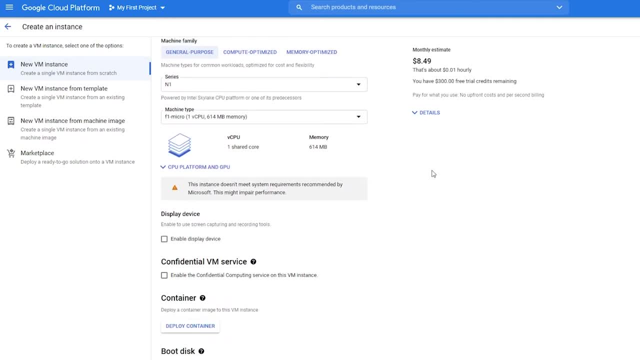 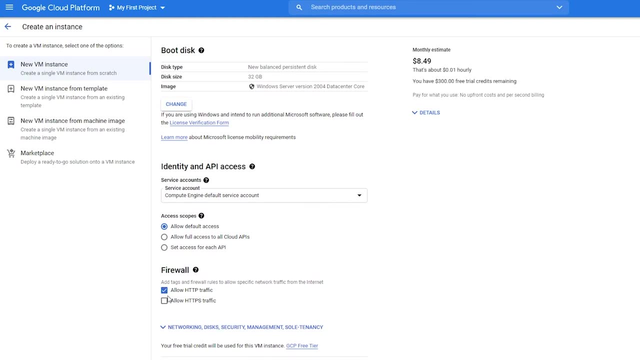 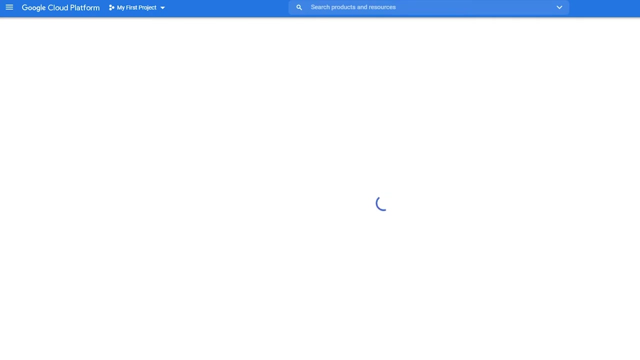 space. so yeah, our cost jumped right now. so now, from over here, what i want you to do is that i want you to scroll down even further and then i want you to check: allow http and also allow https. so now your instance is going to be created and you will not be charged unless you allow to do so. 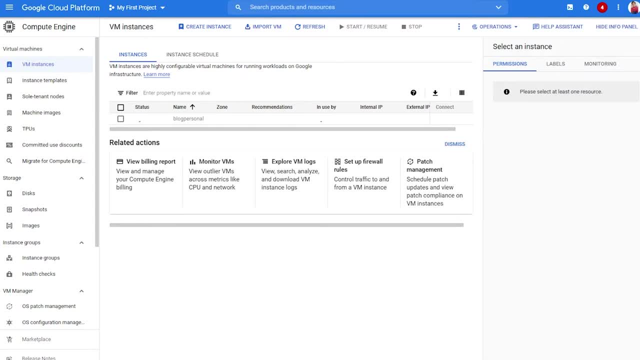 basically, you will be given a 31 day free trial. guys, that is insane. if you were to consider that you were being given all the different features of a hosting service all that so quickly and so cheap. now, in my experience, this usually takes about 15 to 20 seconds to set up, but it might. 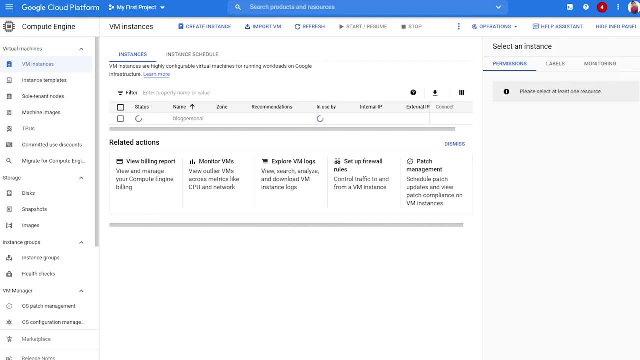 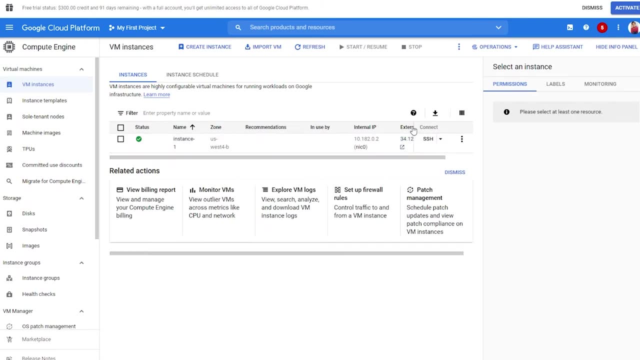 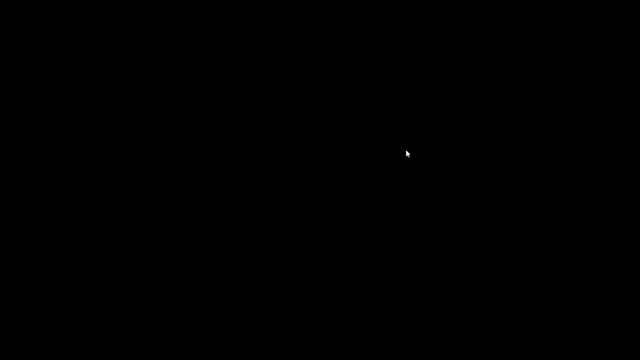 take a bit longer, i don't know why, so i'm gonna simply pause the video for now and i'm gonna catch in just a second. so once this has loaded up, now you will have your external ip, and then you also have your connection address and everything else. so now what you can do is you can simply copy your 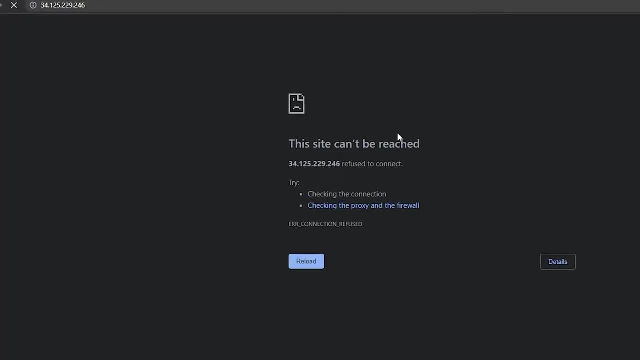 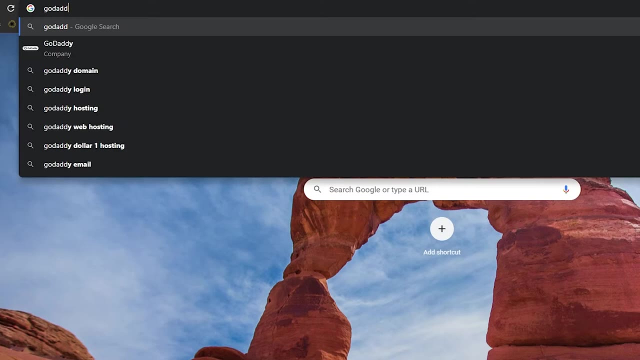 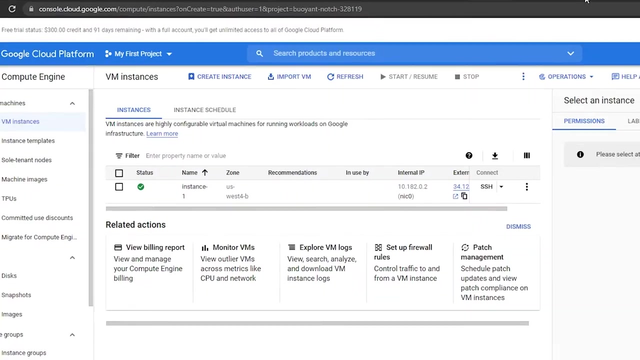 external ip and then you can simply share that with your domain provider. this is going to be your external ip. you can simply copy it and then, for example, if you were to go to godaddy or like you know any other domain provider, whichever one you use- you can simply give them your external ip. 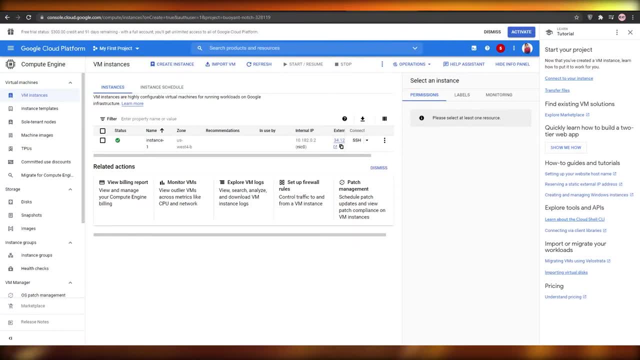 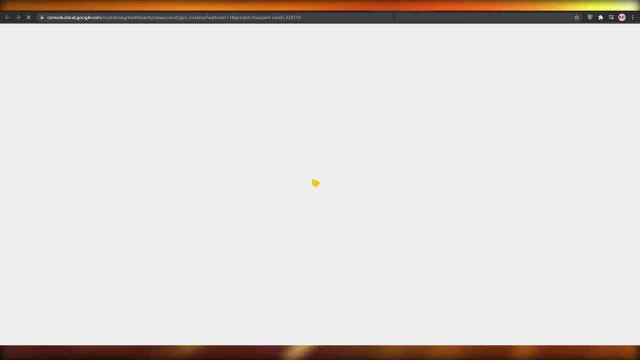 they will be able to link your domain with your particular vm machine. so, like it, is that that simple. so now what you can do is you can actually monitor your vms as well. so, like, what this means is that you can actually see how many people are coming onto your website and how many people are. 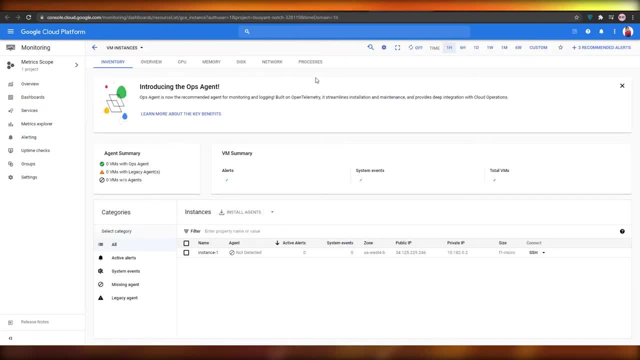 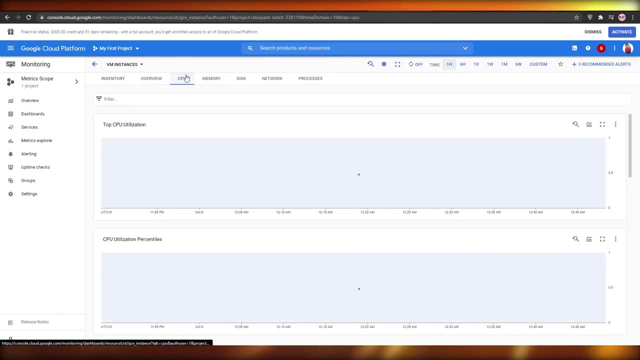 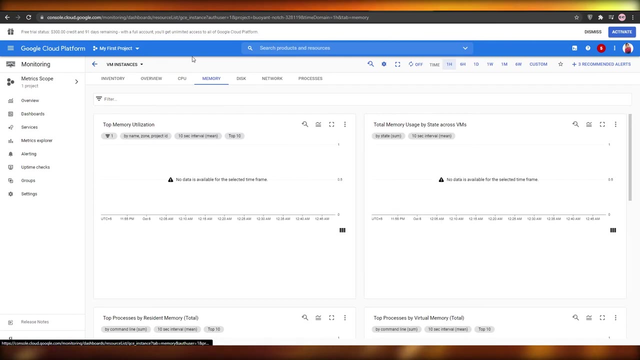 staying onto on your website and do you need to upgrade your website or anything? so yeah, all of those things can be tracked via this particular tracker. so over here you can see your cpu usage. your server starts to be a bit slow. well then, i would highly recommend that you guys upgrade your. 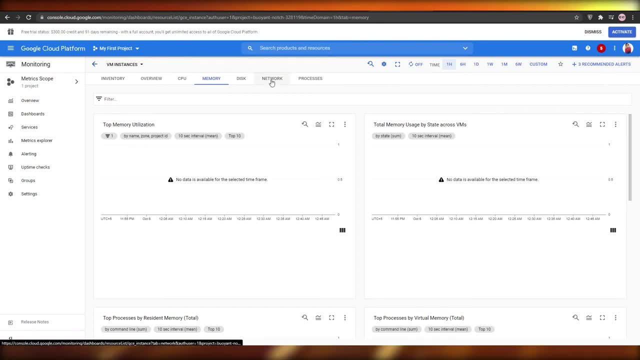 cpu and your memory. and then for example, let's say, if you want to add more data like videos and stuff like that, well then for that you will have to upgrade your disk storage as well. but that can be done later on, you don't have to necessarily do it right now. and then also you have other features. 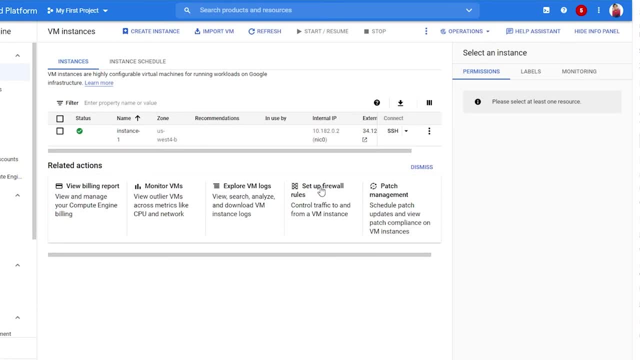 as well. so you can also set up firewall rules as well to keep your server as secure as possible. and then also you can view the website as well. so you can also set up firewall rules as well to keep your server as secure as possible. and then also you can view the. 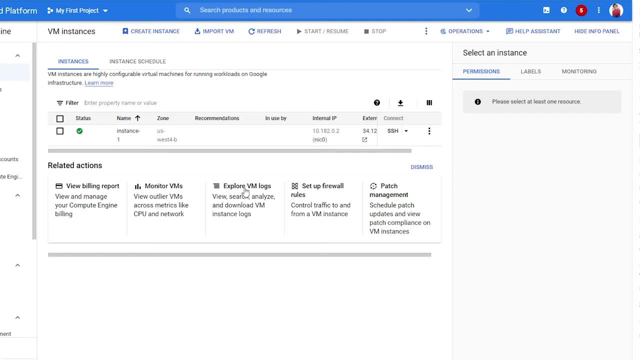 virtual machine logs as well to see if there is anything suspicious going on, to see if any hacker is trying to hack your blog or something. you can see all of those things in your logs and then also you can patch your server if you see anything is not right or if you want to basically upgrade your 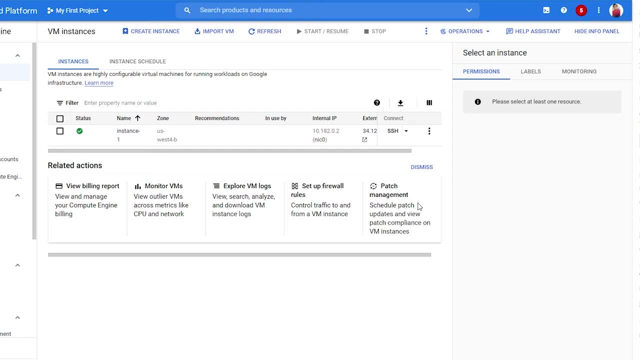 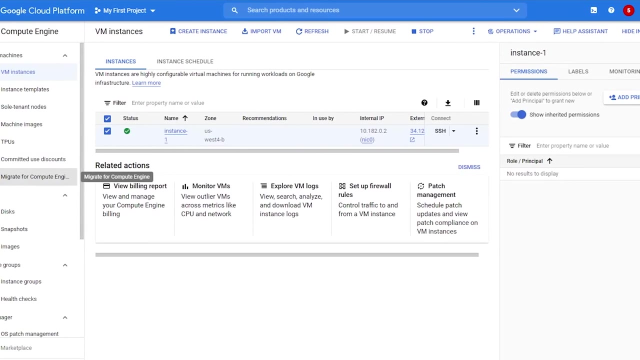 security. you can do all of that using the tools over here, and then maybe, if you want to, like you know, decommission your server, you can simply click on these three buttons and click on delete and your server is gonna be deleted. now you can even add labels. you can do a lot of things, and then, from the left side, you have a ton. 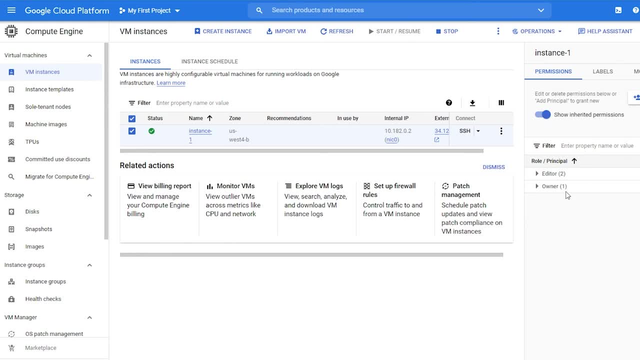 of options that you can explore on your own, but this is how you can essentially grab yourself a free website off google cloud, all for absolutely free, and then later on, if you want to, like you know, go pro, well then you can definitely go pro, and then you can actually pay the five dollar and 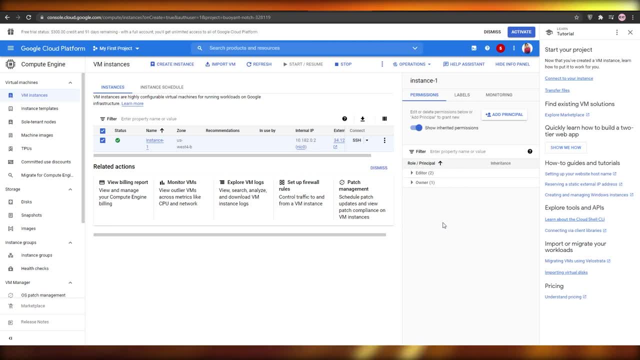 that is going to be money well spent, because it is not that expensive and the facilities you are getting. they are far beyond capable. so, guys, this was the video, and if this video helped you out, make sure to smash that like button. subscribe until next time, goodbye.